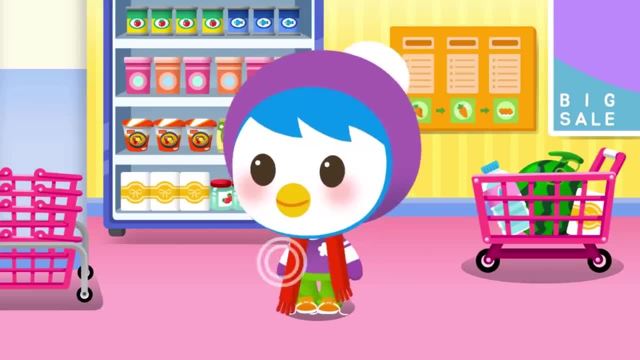 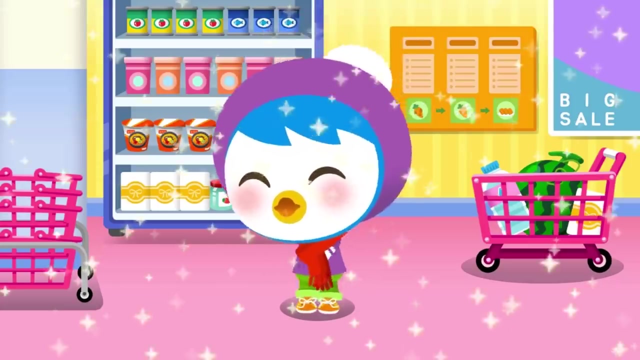 Eek, Let's change Petty's clothes to something safer. A long scarf can get caught between the steps. Overly long pants can make you stumble and fall. A loose shoelace can get caught between the steps Outstanding. Petty's clothes are now safer. 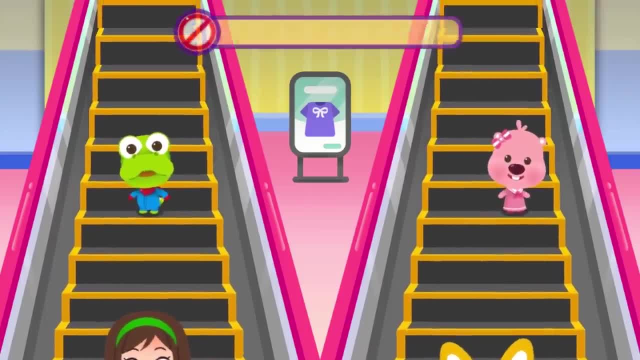 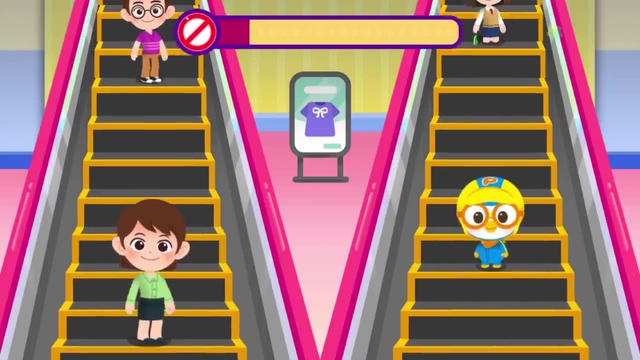 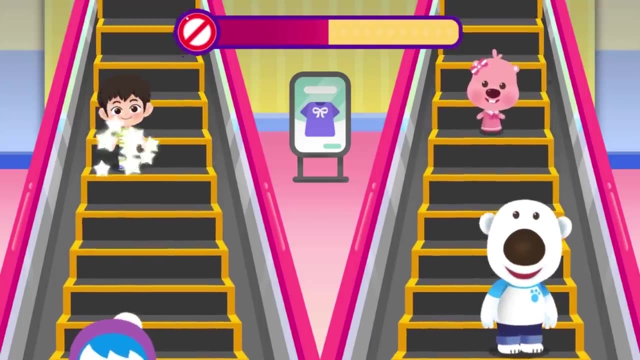 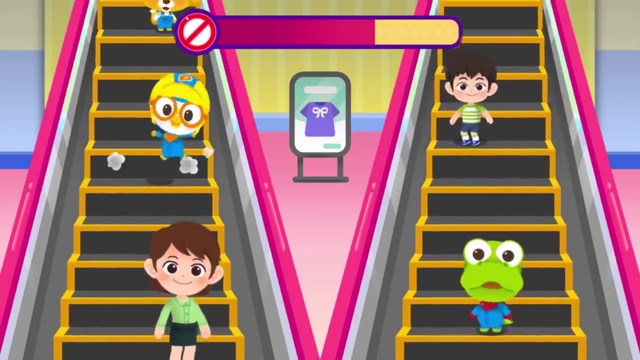 Spot the friends who are being dangerous: Eek, It's dangerous to run around. It's dangerous to sit on the steps. Not holding on to the handrail is dangerous. It's dangerous to jump on the steps- Eek, It's dangerous to run around. 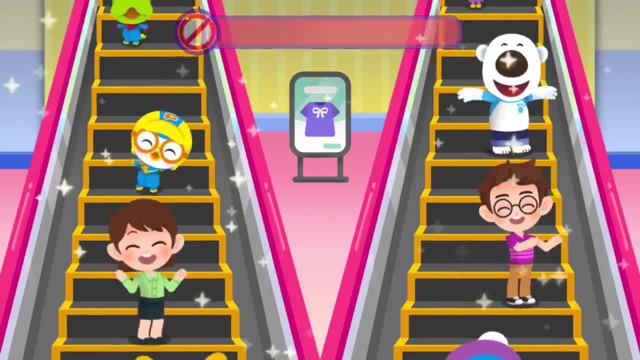 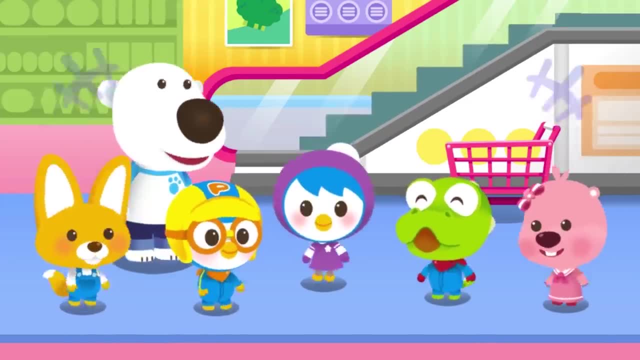 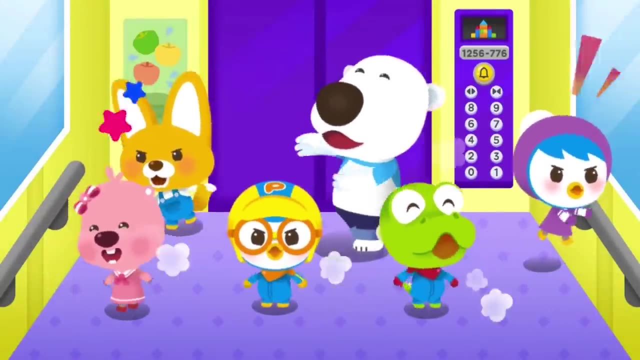 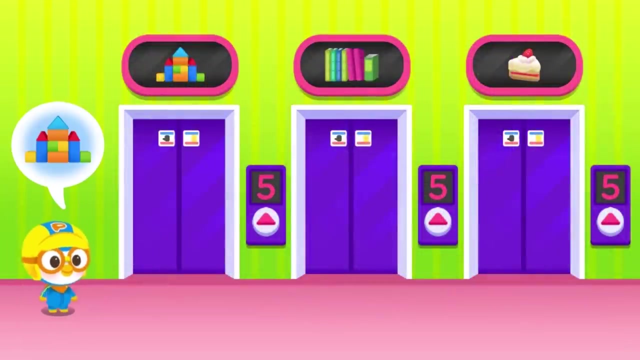 It's dangerous to sit on the steps. Good job, The friends all rode the escalator safely. Always remember escalator safety. It's dangerous to play and run around in the elevator. Let's learn about elevator safety. Choose an elevator for Pororo. 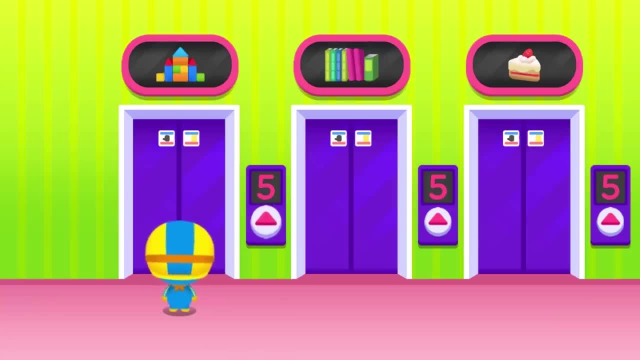 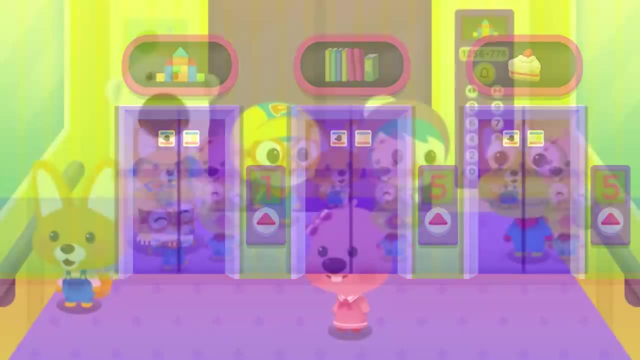 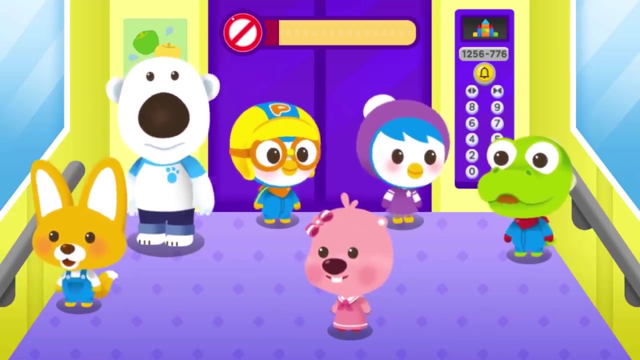 Press the button. The elevator is here. Good to see you, granddaughter. Hello, Spot. the friends who are being dangerous Stand still and don't goof around. It's dangerous to lean on the door. It's dangerous to climb on the handrail. It's dangerous to jump in the elevator. 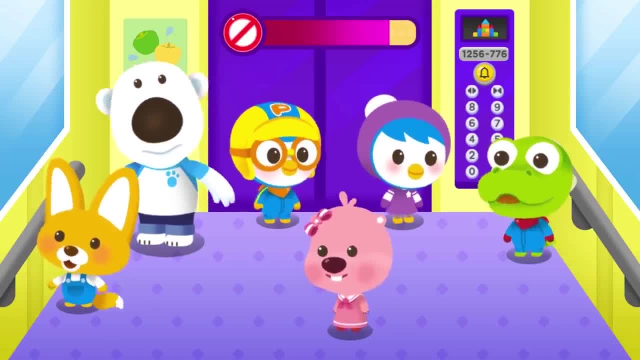 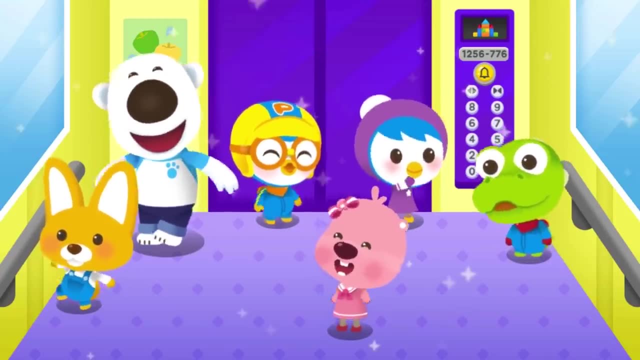 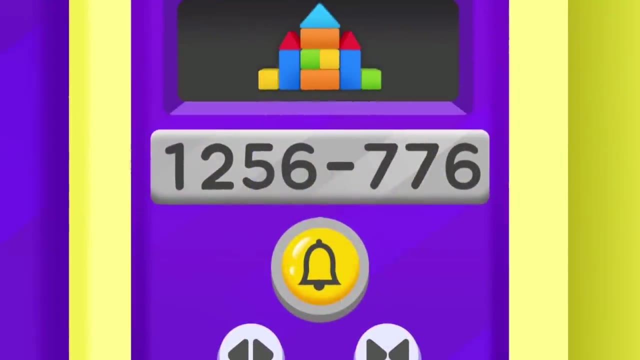 Playing around with the buttons can break the elevator. No, Don't force the door open. Good job, Don't goof around in the elevator. The elevator is stuck. Find a safe way to escape. Call for help with the emergency button. Hello, Read the elevator serial number. 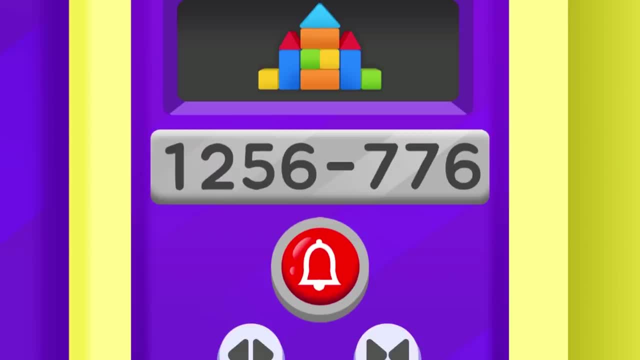 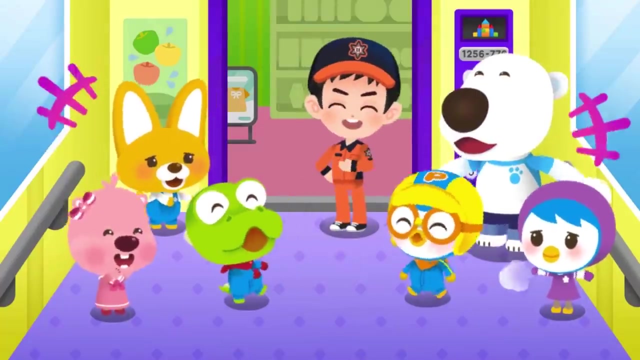 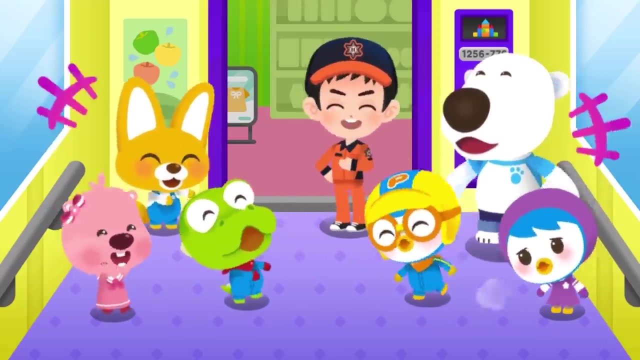 for a quick rescue, Press the buttons to match the serial number One, Two, Five, Six, Seven, Seven Six. Okay, We are on our way. Hold on Phew. The friends are all safe and off the elevator. Always remember elevator safety. It's dangerous to wander off alone in the supermarket. 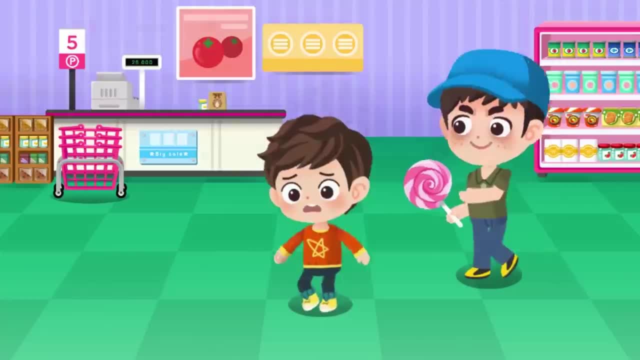 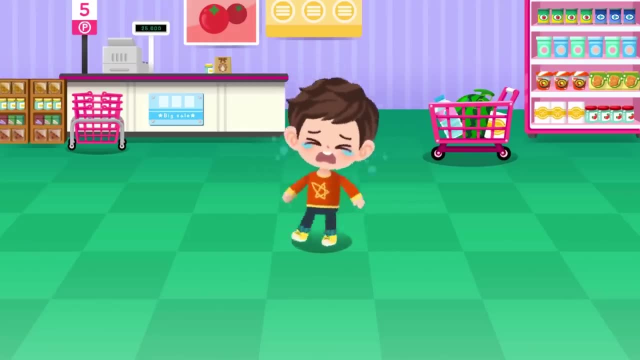 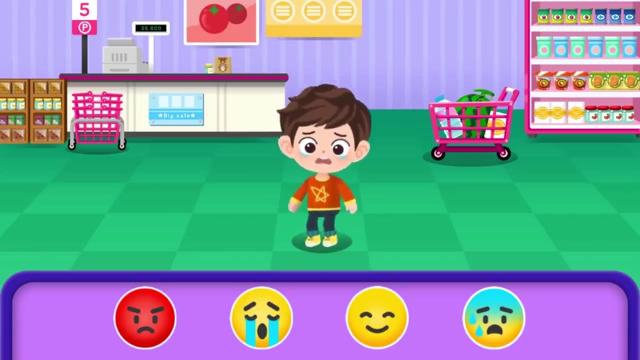 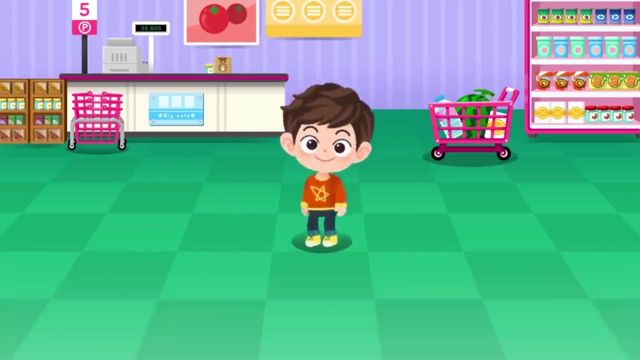 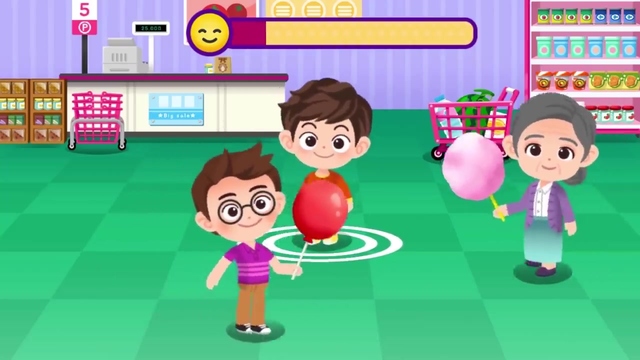 Let's learn about lost child safety. Mom, Dad, First, be calm and don't cry. Find the happy face. Don't wander off, Stay still until your parents find you. La, la, la, la, la, la, la, Wow, No, Wait in place. 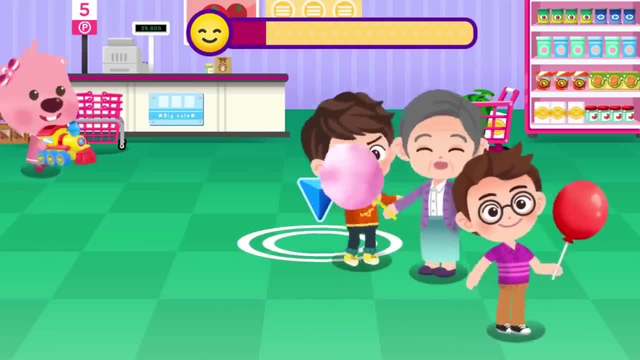 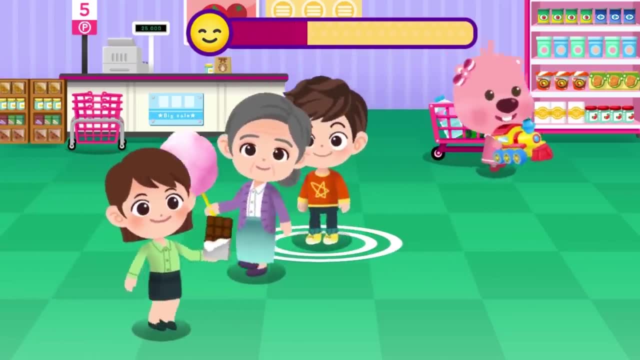 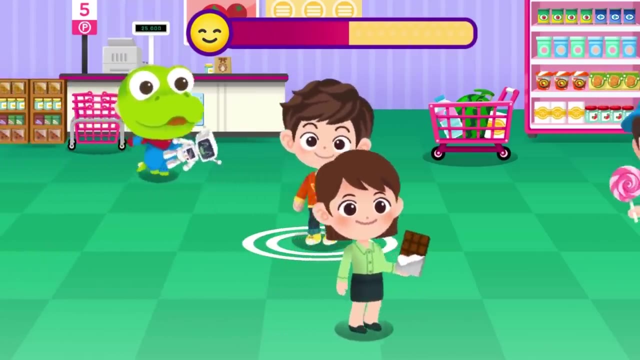 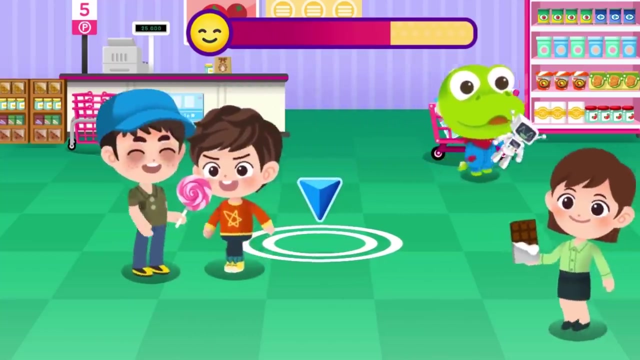 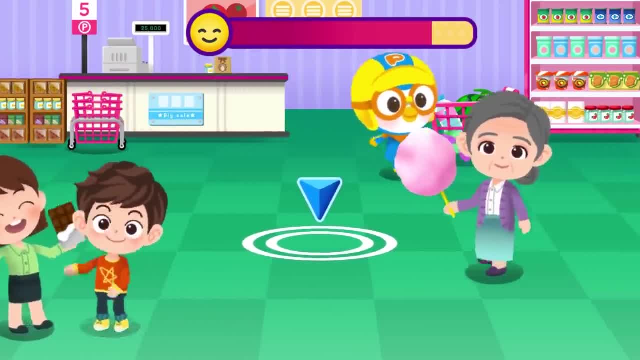 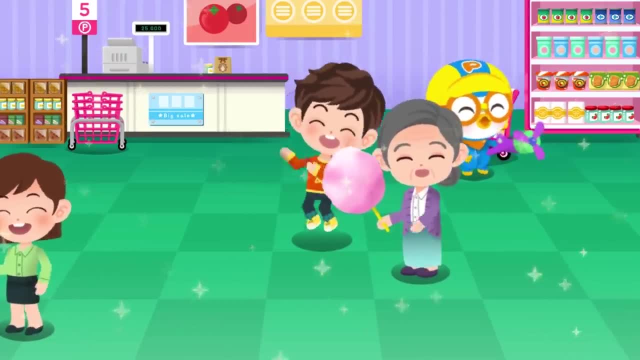 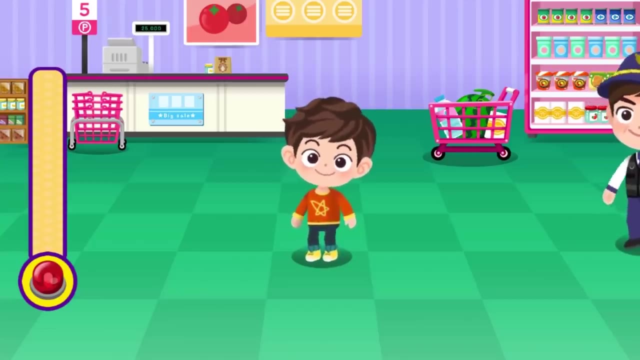 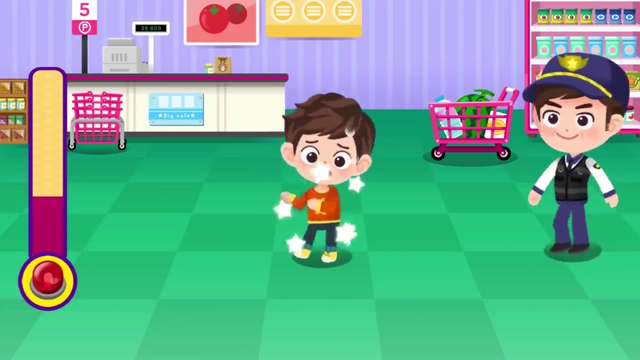 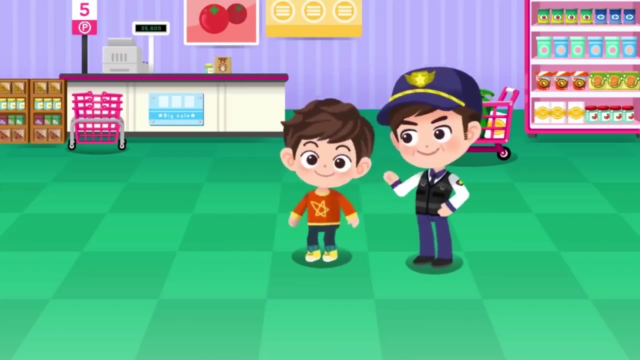 Hi, hi, No, Wait in place, Good job. Don't wander off. when you get lost, Ask for help from an adult. Tap on Diri to call a policeman. You can do it. Help, Please help me. Hi kid, Are you lost? 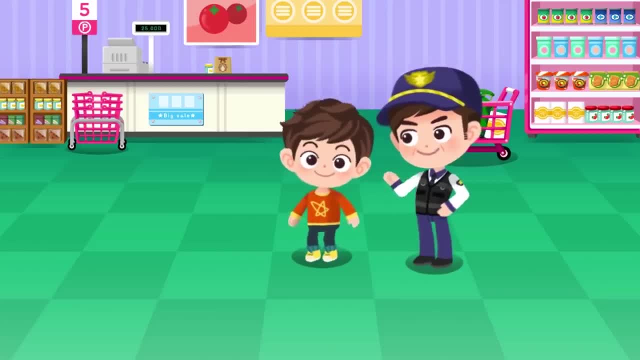 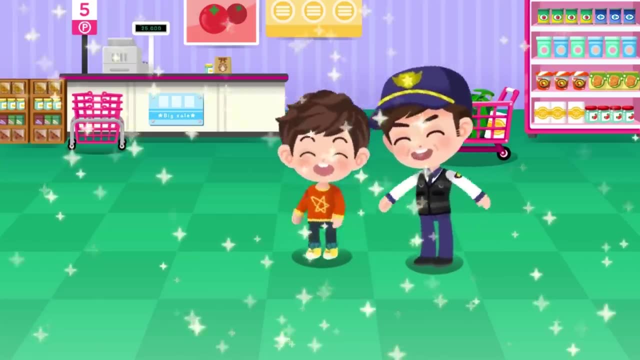 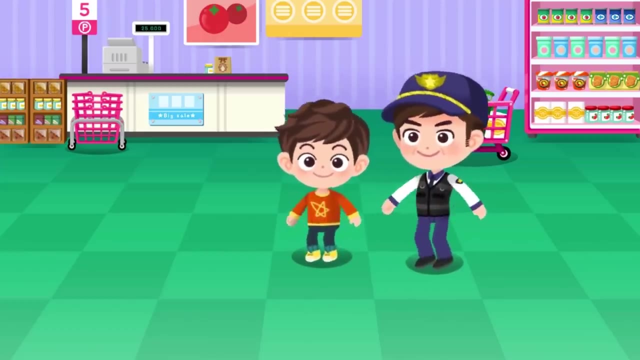 Let me help. Do you know your parents' phone number? Yes, I know their phone number. Ha ha, ha, ha ha. Remember important information like yours and your parents' names and phone numbers. Swipe on the word bubble and reveal the phone number.